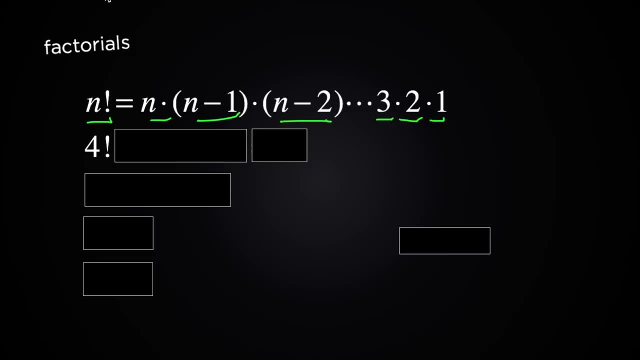 So I'm just going to give you a few examples here. Four factorial is equal to four times three times two times one, which is equal to 24, and two factorial is equal to two times one which is two, and one factorial is one. And what about zero factorial? 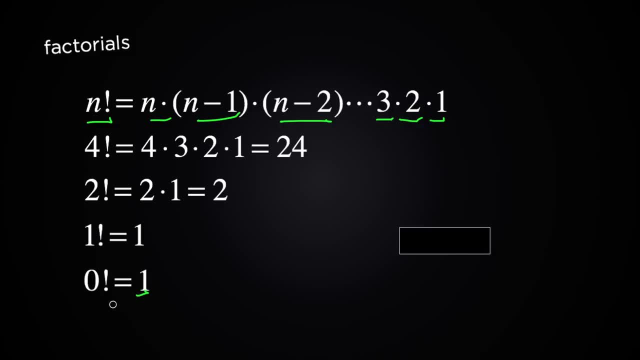 It's actually defined to be one And you might say: why is that? But you know, basically it's a very simple question. It's actually defined to be one And you might say why is that? But you know basically. 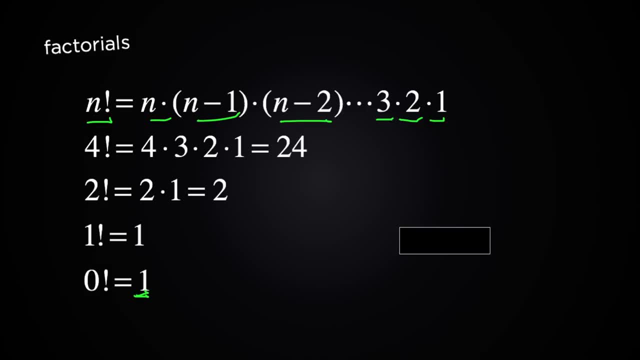 that's just how it's defined. And let's just say: here we're trying to write a function called, let's say, fact, which takes a positive integer or zero as its argument and returns the nth factorial. And let's say we want to write this function using recursion. How can we do that? 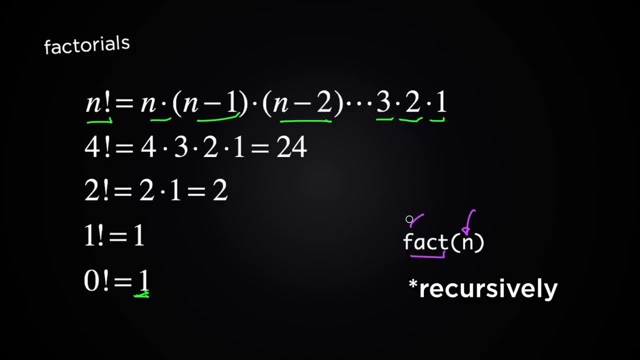 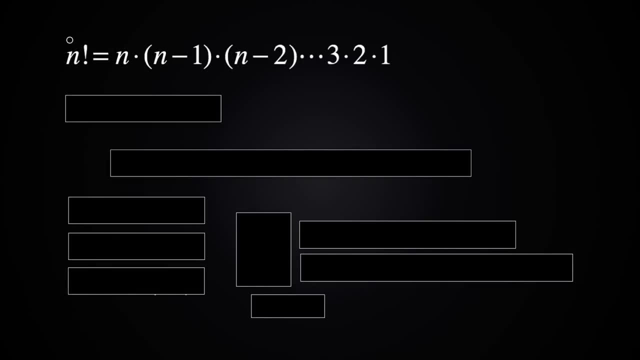 To solve this problem or to write this function recursively. we need to actually examine this equation in a little bit more detail. Okay, So I brought that equation, So I brought that equation over here And, like we saw earlier, we had n factorial being equal to n times n minus one times n minus two. 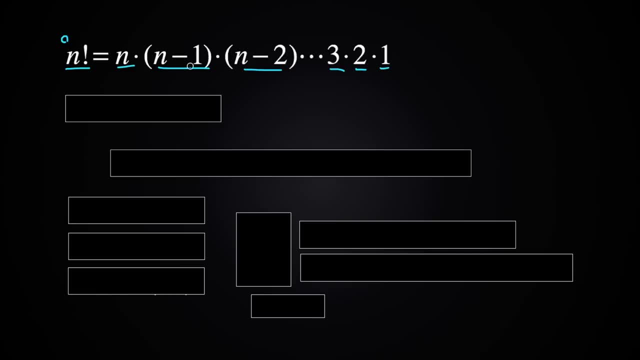 and so on, times three, times two times one. And when you see this equation and when you look at this part following the first n, you might notice that this part is equivalent to n minus one factorial, And that might be more obvious if I write it separately here as n minus one. 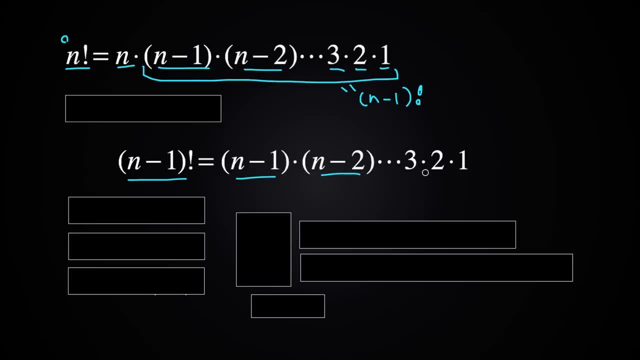 factorial equals n minus one times n minus one factorial. So this whole thing is equivalent to this part. So you might say: well, we can rewrite n factorial as n times n minus one factorial, And that's good. This new equation is mostly correct. 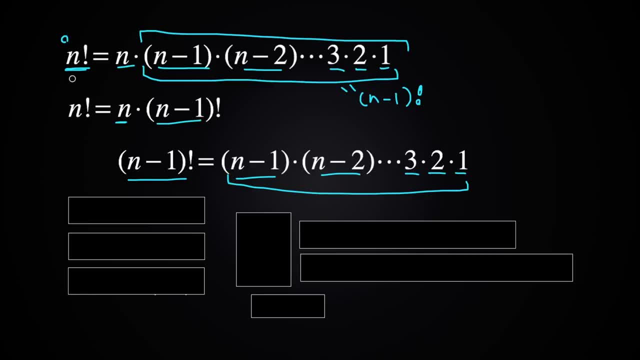 but it's not a complete definition of factorials. Let's see why. Let's say: if you plug in two to n right here, it works just fine, And then you can see that it's not a complete definition of factorials. It's just fine because you'll get two factorial being equal to two times two. 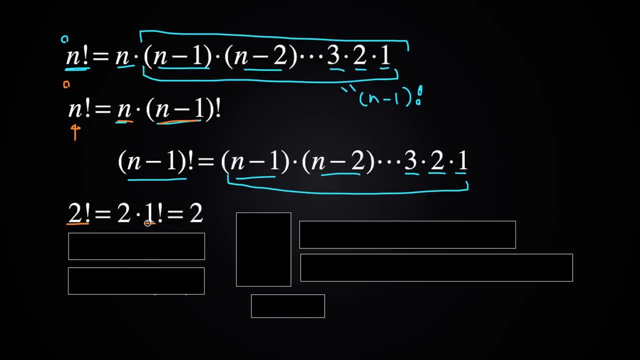 minus one factorial, which is one factorial, and one factorial is one. So two times one factorial is two. And that's correct. What if you plug in one here? It's still good, because you get one factorial being equal to one times one minus one factorial. 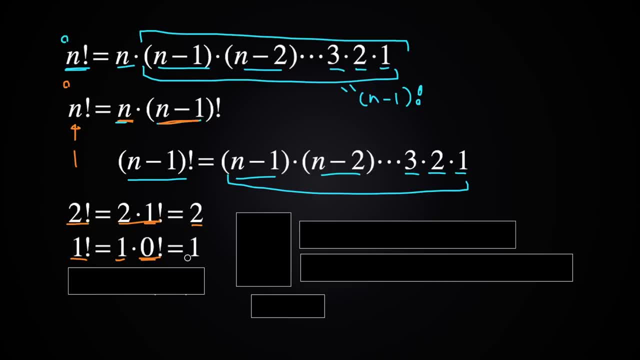 which is zero factorial, and zero factorial is one, As we saw earlier. so that's one and this is correct. But as soon as you plug in zero here, it breaks. Let's see how that works. Zero factorial is equal to zero here. 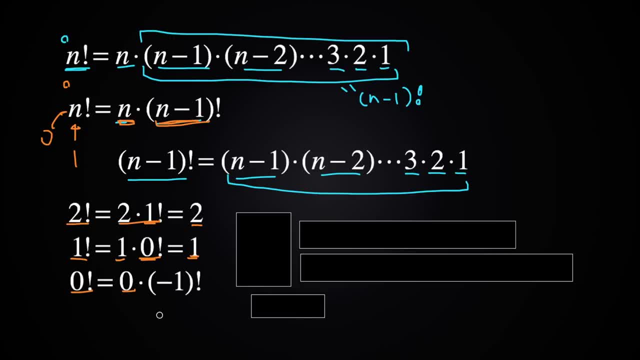 right here times zero minus one factorial, which is minus one factorial and minus one factorial is not defined. So this definition works only for n that is greater than or equal to one, but it doesn't work for zero. So actually for this definition, 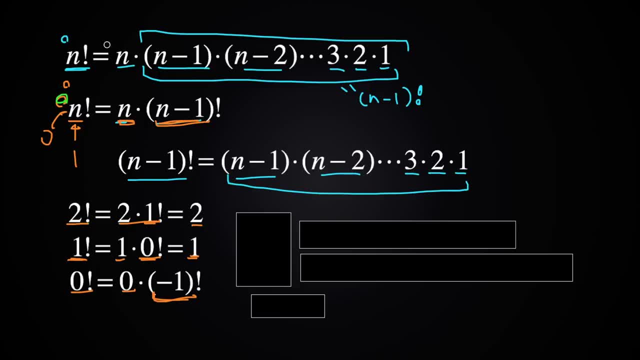 it's not a complete definition of factorial, but it's a definition to be complete for factorials We need to write n factorial as two separate cases. So here we're going to write: n factorial is equal to n times n minus one factorial. 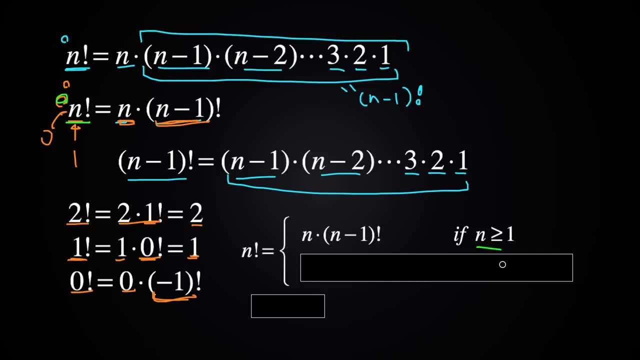 if n is greater than or equal to one, And if that's not the case, or if n is equal to zero- I wrote otherwise here- n factorial is equal to one, And this is actually a complete definition of all factorials. for all positive. 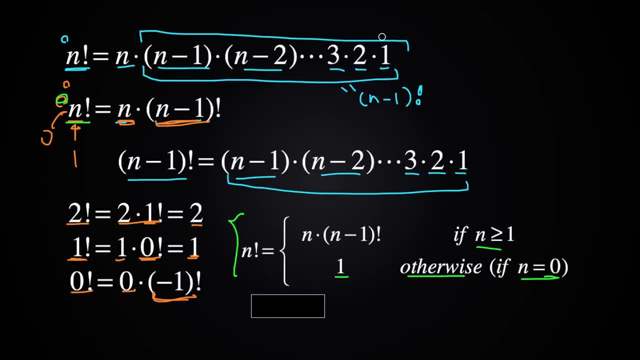 negative, positive integers and zero. So let's just quickly see how we can use this new definition of factorials to find the factorial of any positive integer, Let's say three. So if you ask yourself what's three factorial, there are two ways of answering that question. 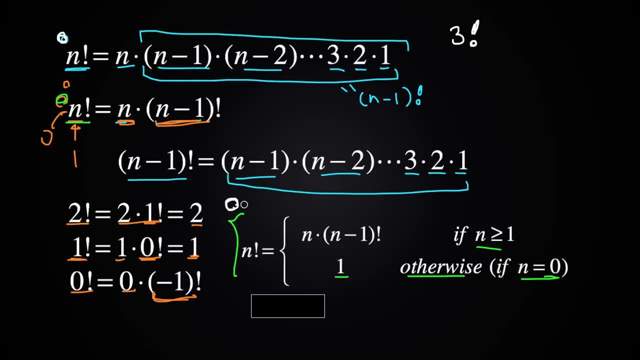 The first one would be to use the old definition, And then the second way would be to use this new definition- And let's use this new definition here, because we're going to use this new definition later to to write a function using recursion as well. 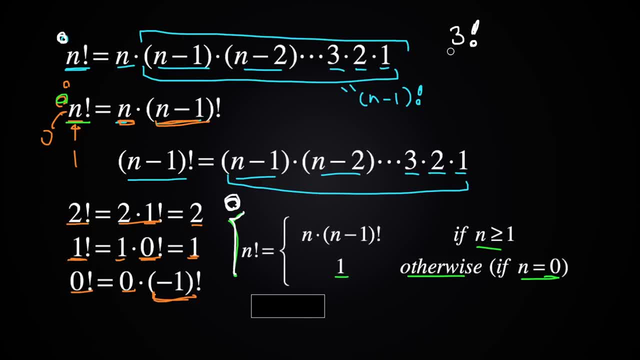 So, using this definition, we can ask ourselves: what's three factorial? Well, three is greater than or equal to one, So by definition, this is equal to three times three minus one factorial, which is two factorial. And then we can ask ourselves: what's two factorial by definition? 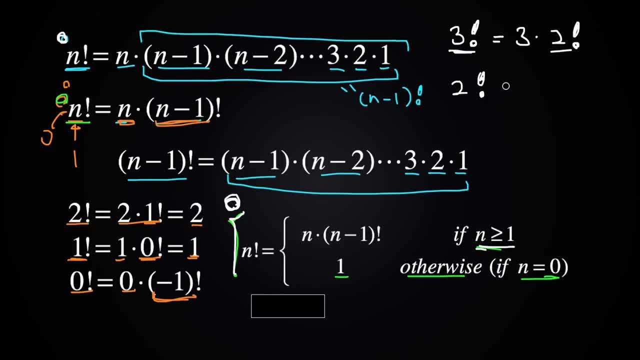 since two is still greater than or equal to one. it's equal to two times one factorial. And then we can do the same thing for one. What's one factorial? Well, it's one times zero factorial. And then, as soon as we have this, 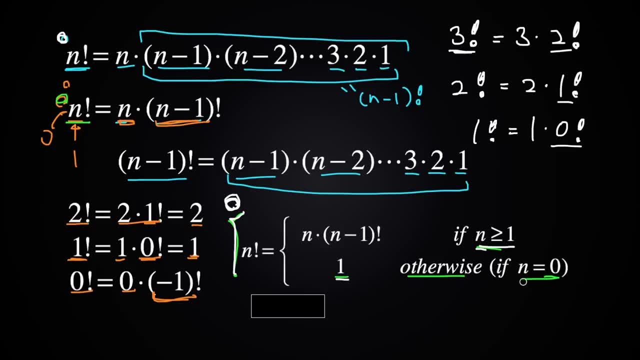 we'll know that zero factorial is one by definition, And as soon as you have that, you can plug one to zero factorial here, And then you'll know that one factorial is equal to one times one, which is one, And then you can plug that back in here. 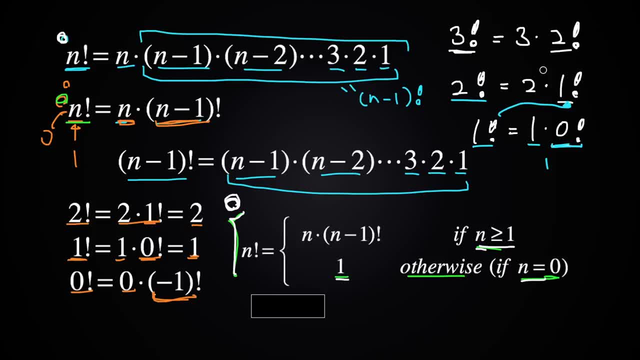 And then you can plug that back in here And then you'll say: okay, two factorial is two times one, which is two. So we can plug that back in here And then we'll say: three factorial is three times two factorial. 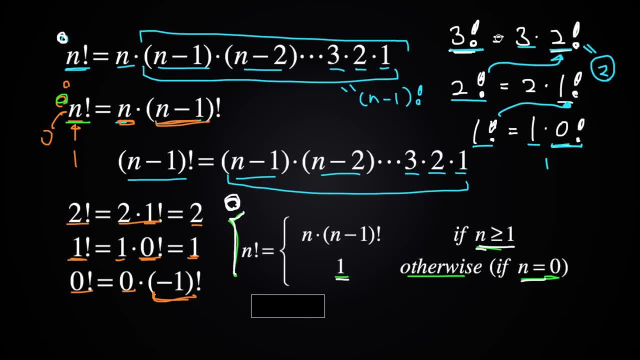 which is two. So the answer here is three. factorial is three times two, which is six. Okay, Now, this whole process might seem a little bit silly, but this kind of thinking is going to be actually the basis for implementing the function we wanted to implement earlier, recursively. 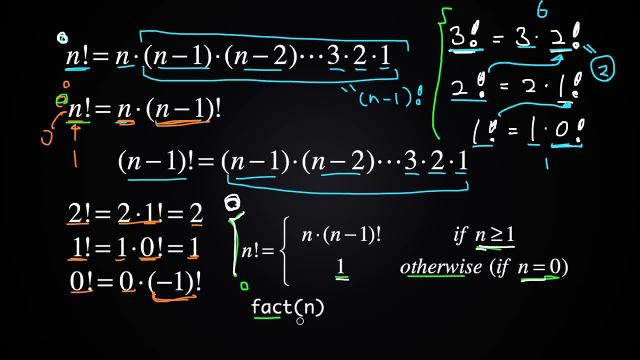 Fact of n. and fact of n, as I said earlier, is going to take n, which is either a positive integer or zero, and it's going to return n- factorial. So let's see how we can implement it using recursion, And actually all you need to do for that is you need to. 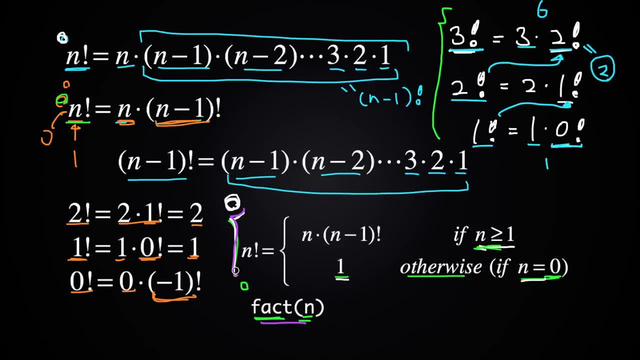 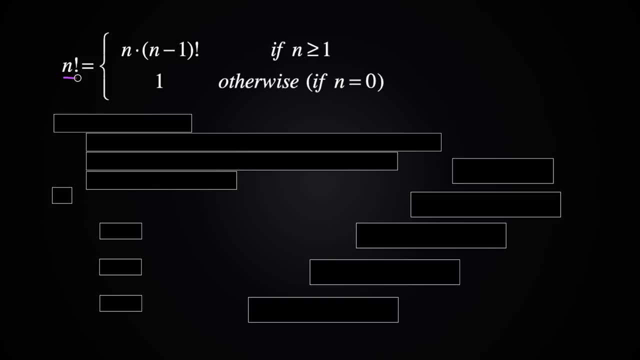 translate this new definition of factorials into code. So let's just bring this definition up here. So, like we saw earlier, n factorial is equal to n times two. factorial n times n minus one factorial if n is greater than or equal to one, and then it's one. otherwise, 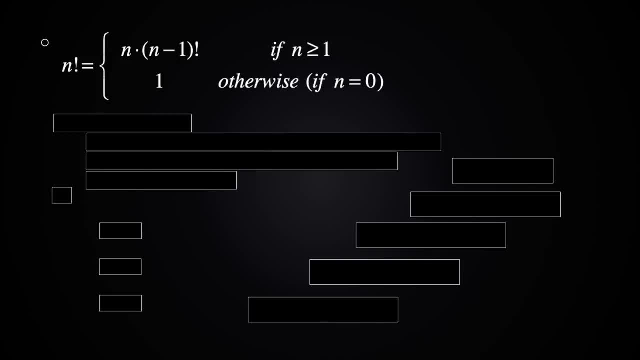 or if n is equal to zero. And then we're going to translate this definition directly into code- And I'm going to use Java here just as an example- And, like we saw earlier, we're trying to write a function called fact which is going to take n, an integer. 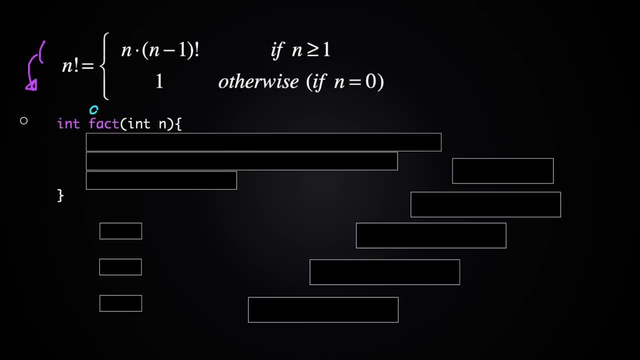 and it's going to return an integer which is going to be n, factorial. And just for simplicity here I'm going to assume that the given n is always positive or zero, So it's never negative, And to write the rest of the function. 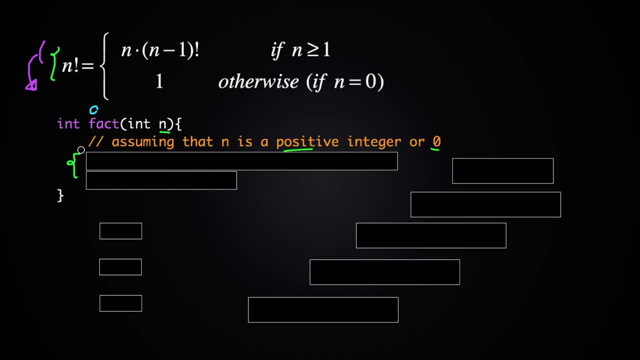 it's pretty simple. We just need to translate this formal definition into code. So here it says: n factorial is equal to n times n minus one factorial If n is greater than or equal to one, And what we're going to return from this function is going to be the value of n factorial. 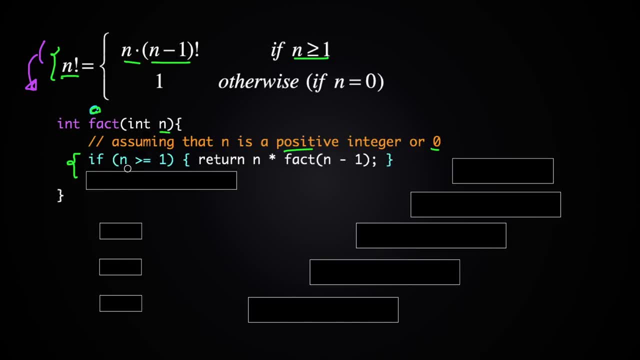 So here we just need to write: if n is greater than or equal to one, we're going to return n times fact of n minus one. So this is the same as saying the value of factorial n is going to be n times factorial of n minus one. 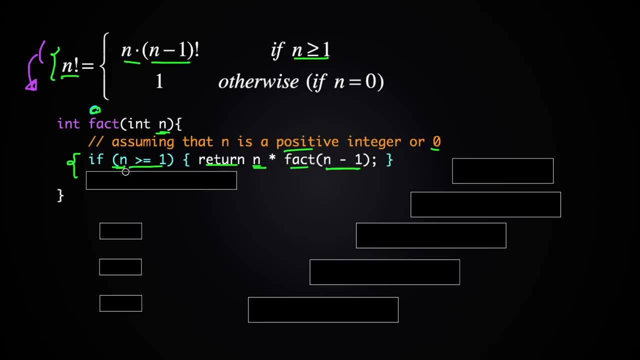 If n is greater than or equal to one, And then we're going to write otherwise, or else- that's when n is equal to zero- We're just going to return one, because we know that that's the value of zero factorial. So, as you can see, 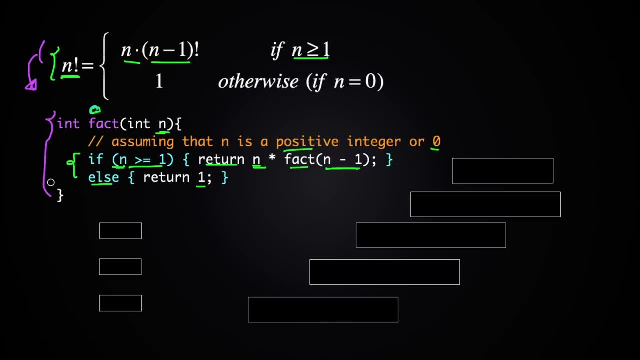 this is a recursive function, Because this calls itself fact, calls itself right here to solve the problem of finding n factorial. Okay, this function seems pretty simple, but does it actually work? Well, it does, to see how. Let's take a look at a few examples here. 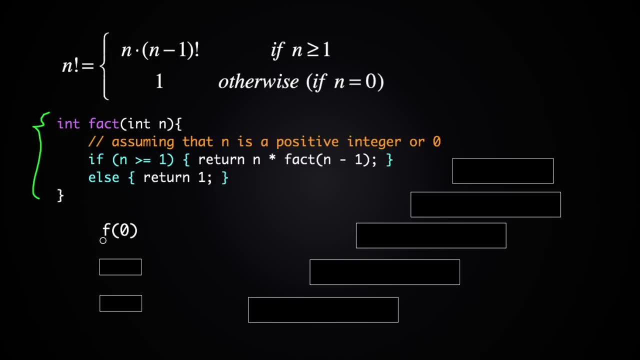 If you have fact of zero, I just wrote it as f of zero. That's pretty easy, because here we get this line right here, because zero is not greater than or equal to one. So we're just going to return one, which is correct, because one is zero factorial. 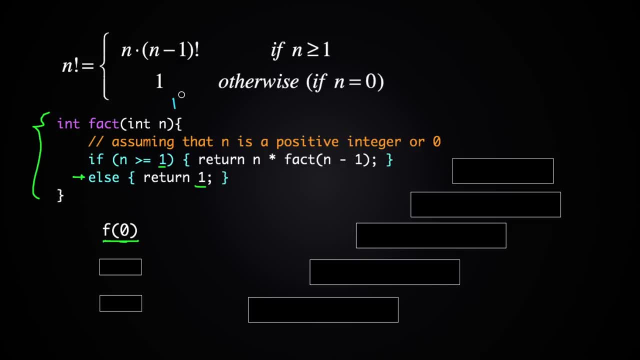 And what if you're given one as n? then I'm just going to write f of one here to stand for fact of one When this is called. it's going to hit this line right here because n is equal to one And then it's going to try to return one times: fact of one minus one. 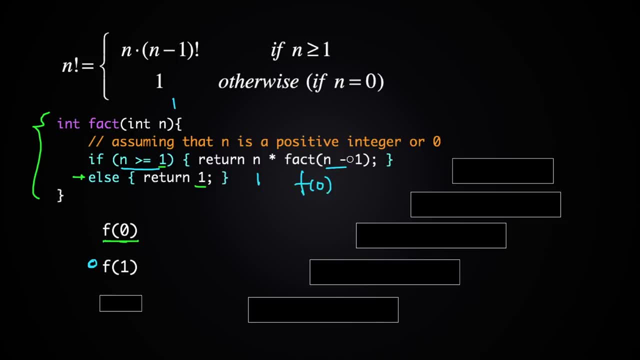 which is zero. So f of zero here. And then when f of zero is called, it's going to go to this right here that we saw earlier. And then f of zero will say, okay, my value is one, So this is going to return one. 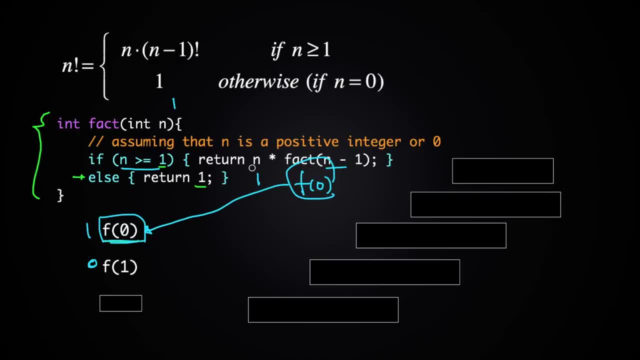 And then, in f of one, it's going to say: okay, well, what I'm going to return is one times the value of fact of zero, which is one. So we're going to return one times one, which is one. 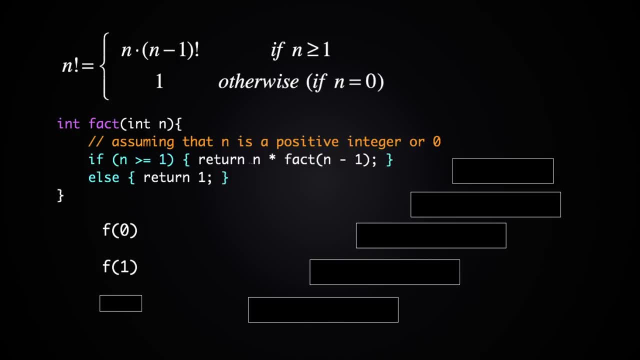 So that's the correct answer. Okay, To help you understand This a little bit better, I'm going to give you another example here. Let's say, fact of four is called- I'm just going to write f of four here. And when it's called, 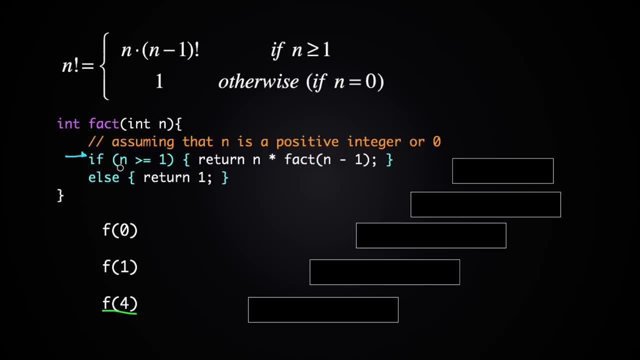 we go to this line right here, And since n, which is four, is greater than or equal to one, it's going to say what I want to return from: that function is four times fact of three. But we don't know what the value of factor of three should be. 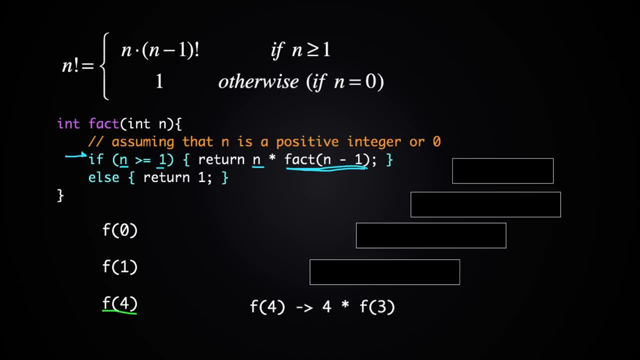 So we need to call that function. So I just wrote it here. Here I'm saying the value of f of four, the return value of f of four, will be four times f of three, And then we need to call f of three to find a return value for that. 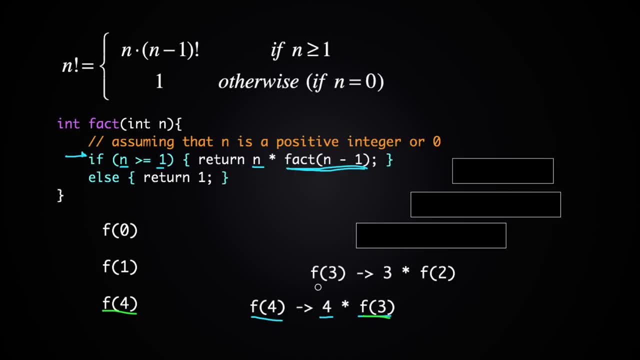 And once we call f of three, the same thing will happen. The return value of f of three will be three times f of two, whatever the return value of f of two is. So we'll call f of two or fact of two. 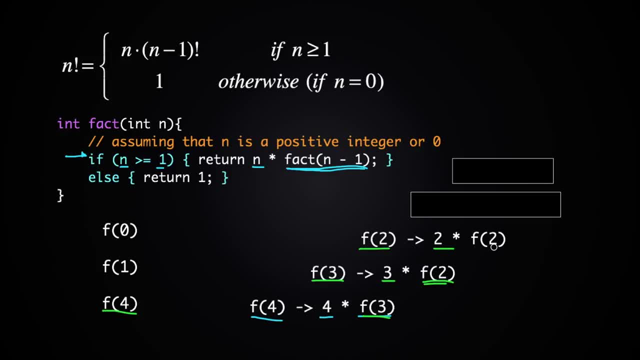 And then we'll say: okay, that's two times f of one. Actually there's a type of here: whatever the return value of f of one is, So we'll call f of one, and then f of one is one times f of zero. 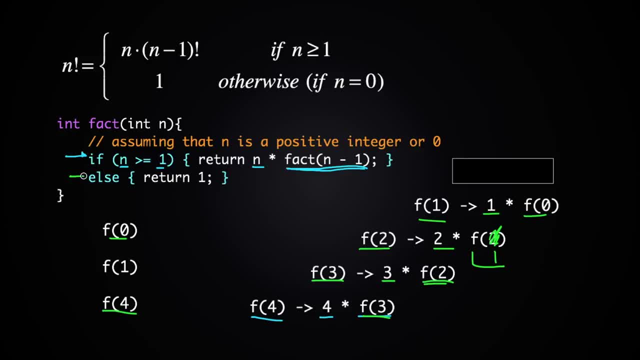 And then, as soon as we call f of zero, we go to this line like we saw earlier. So we'll just return one from that. Once we return one from f of zero, we'll go back to this, call f of one, And then we'll say: 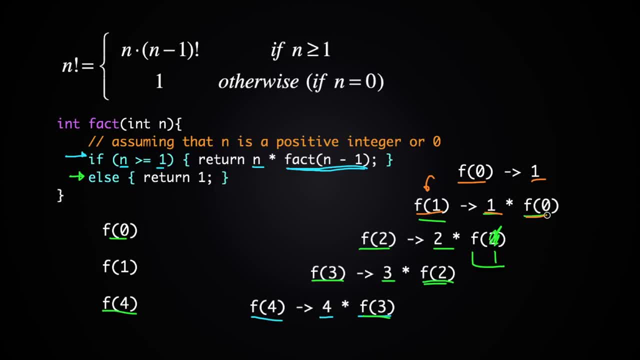 okay, we want it to return one one times f of zero And we now know the value of f of zero, which is one. So we'll just say we're going to return one times one, which is one, from this function. 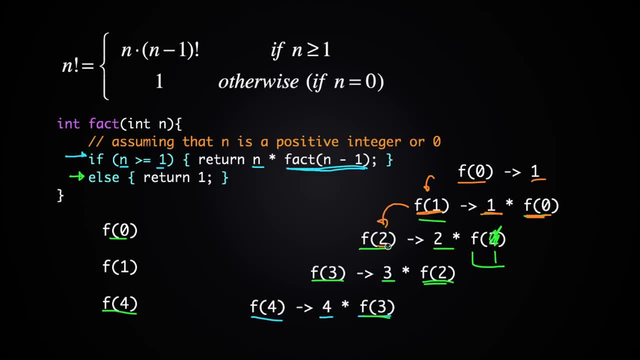 And then we'll go back to this call where n was two And we want it to return two times f of one, whatever the return value of f of one was, And that turns out to be one, So we'll return two times one. 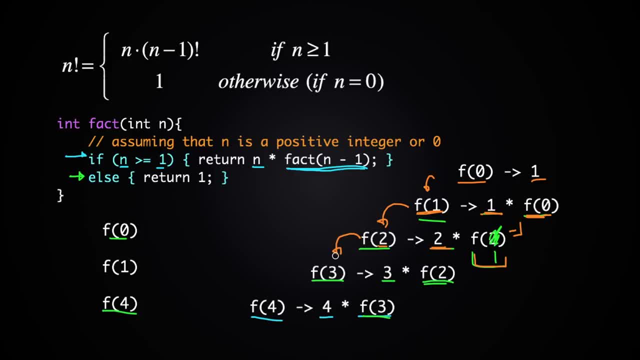 which is two from this function, And then we'll just basically keep doing that. f of three wanted to return three times f of two, And f of two happens to be two here, So we'll return six right here And then we'll go back here. 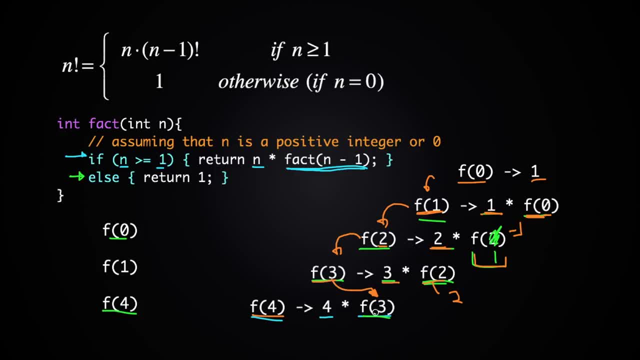 the original call that we made, And then f of three turns out to be six, So we'll say, okay, f of four, we want it to return four times, whatever the return value of f of three, which turns out to be six. 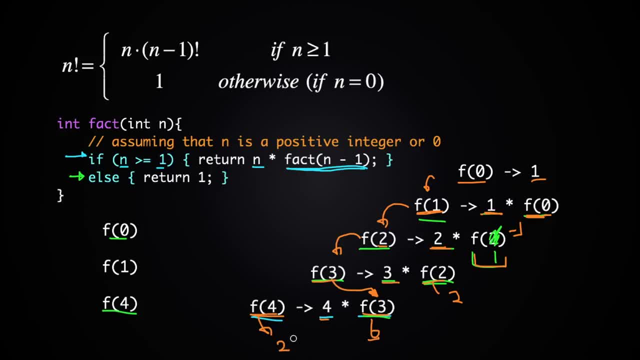 So we'll return 24 from this function, which is correct. And this wraps up this section about factorials. Let me know in a comment below if anything was unclear. Okay, now to better understand recursion, let's take a look at another example here. 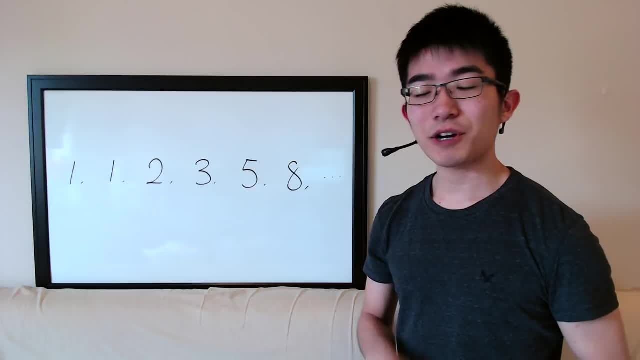 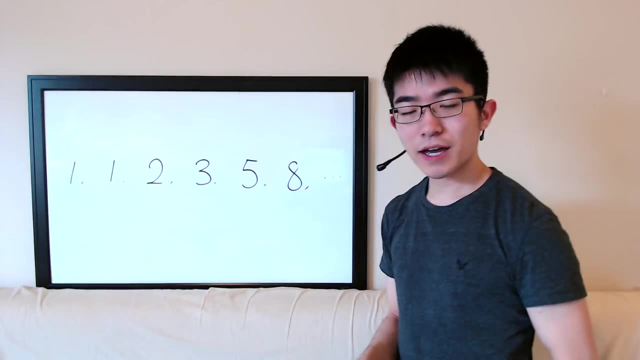 the Fibonacci sequence. So I already talked about this in one of my previous videos. but the Fibonacci sequence is a sequence of numbers that starts with two ones at the beginning, and the numbers after that are generated by adding up the two previous numbers. So, for example: 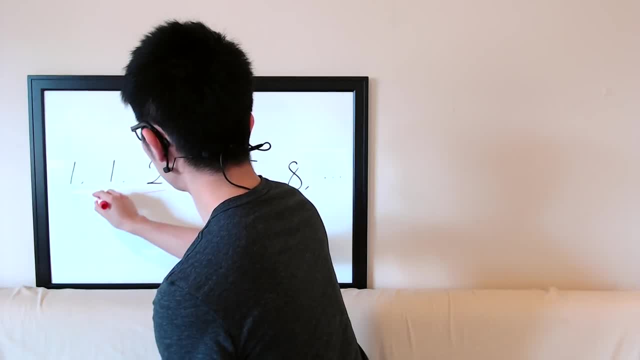 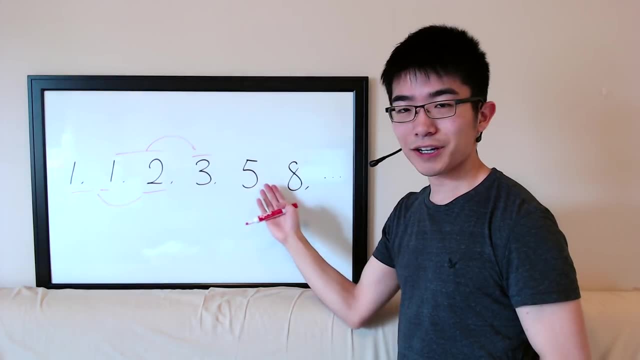 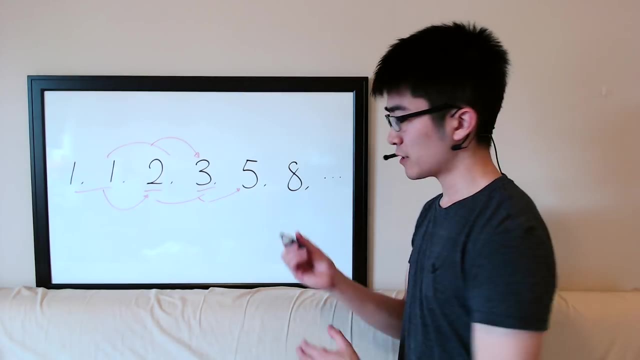 the third number is two, because one plus one equals two, And then the fourth number is three, because one plus two equals three, and so on, and then it just keeps on going forever. And given this sequence, let's just say that we're trying to solve the problem of writing a function. 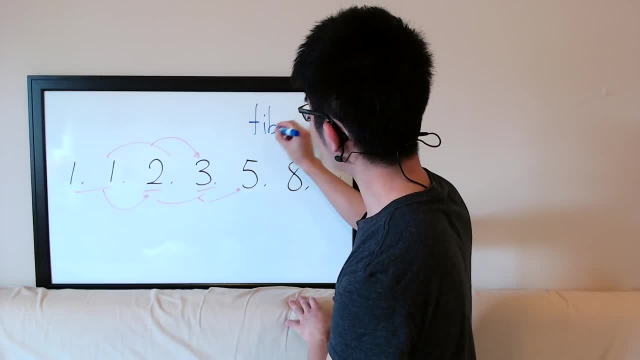 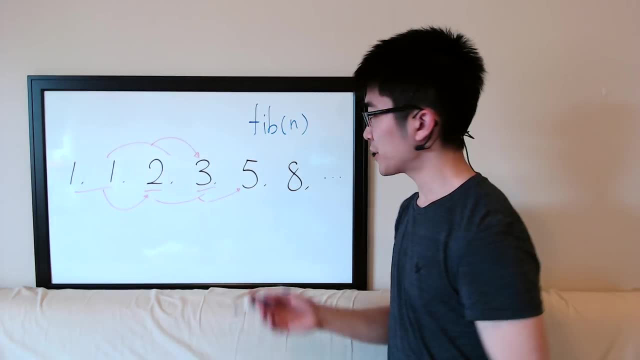 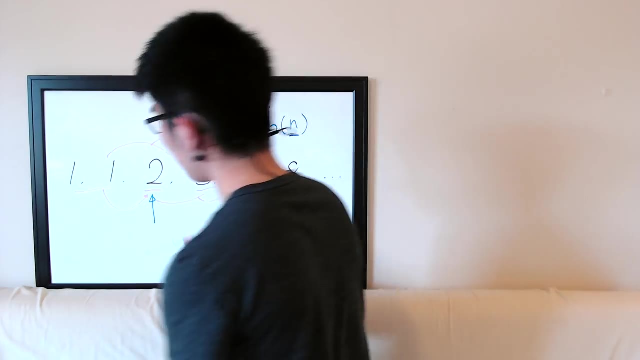 let's say Fib, which takes a positive integer n and returns the nth number in this sequence, the nth Fibonacci number. So if you're given three as n, in this function you should be able to find and return the third Fibonacci number, which is two. 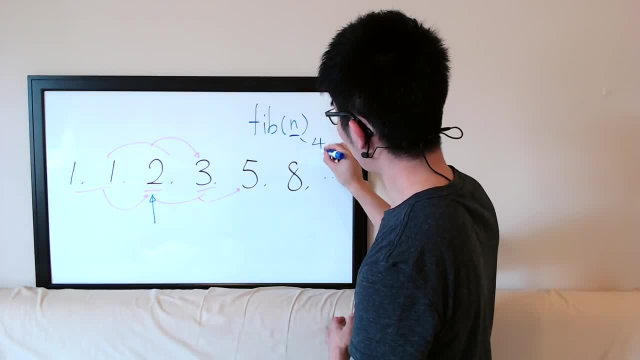 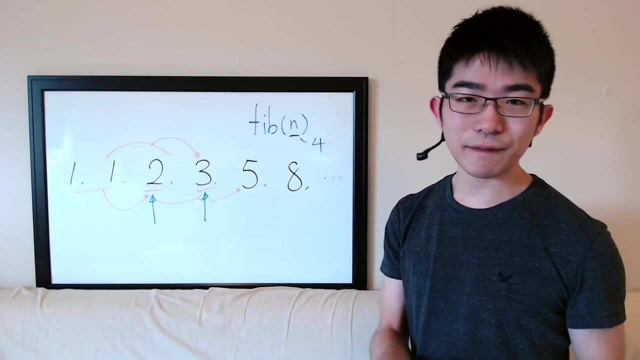 And if you're given four as n, you want to be able to find and return the fourth Fibonacci number, which is three, right here Now. if you want to try solving this problem yourself, pause the video right here and post your solution in a comment below. 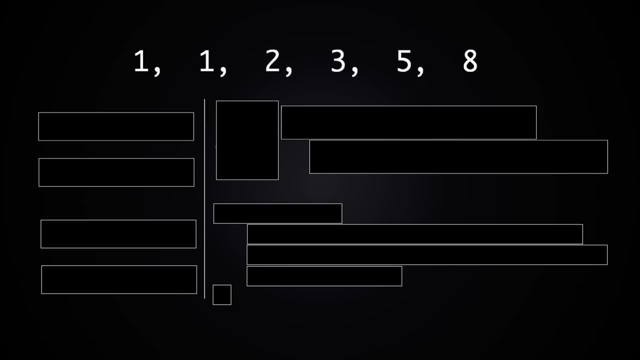 if you want to share it with others. Now, to solve this problem using recursion, you need to first form the Fibonacci numbers and then you need to define the relation between different Fibonacci numbers, just like we did with factorials. So for that we're going to write: Fn equals Fn minus one plus Fn minus two. 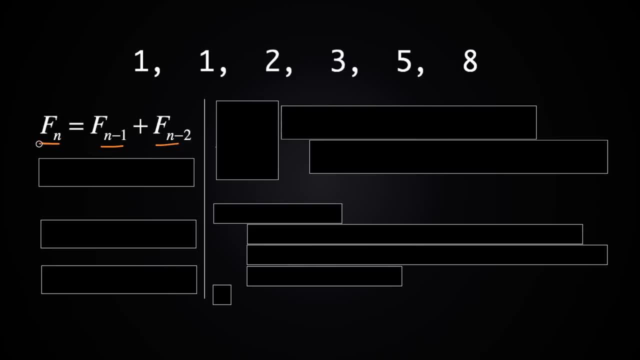 So I'm denoting the nth Fibonacci number as Fn, And this is saying the nth Fibonacci number should be the sum of the two previous Fibonacci numbers. So an example here would be this one right here: F5 equals F4 plus F3. 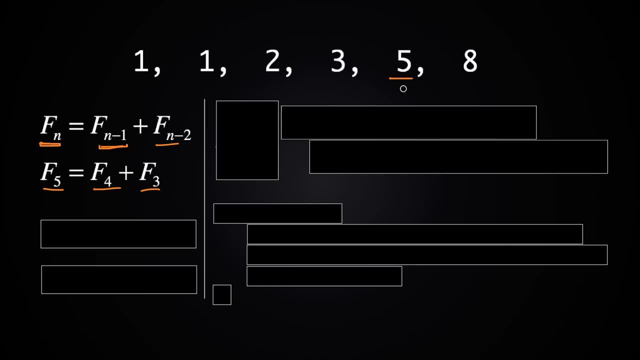 So the same. The fifth Fibonacci number, F5, right here, should be the sum of the fourth Fibonacci number, this one right here, plus F3, which is this one right here. So just like we saw in the case of factorials. 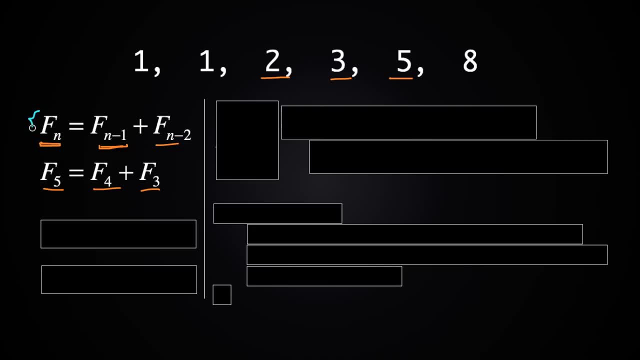 this equation is correct most of the time, but it's not complete. So if you plug in five to n, it's correct. This equation is still correct. But as soon as you plug in two to n, you get F2 equals F1 plus F0.. 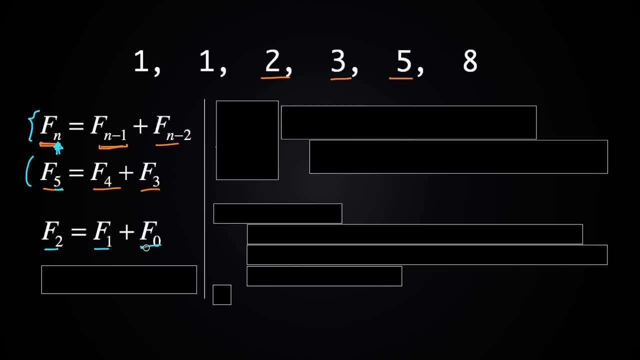 And here I didn't define F0, zeroth Fibonacci number, I guess. So this equation just breaks And it's the same thing if we plug in one. here We have F1 equals F0 plus F minus one. F1 is the first Fibonacci number and F minus one is not defined. 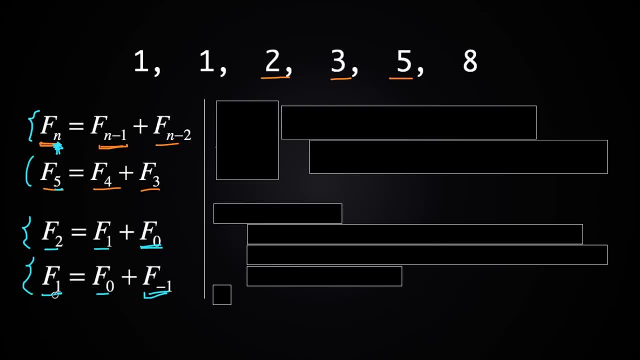 So this equation doesn't work for n equals one either, And to fix this equation we need to actually rewrite it as two parts. The first part is going to be just like we saw: Fn equals Fn minus one plus Fn minus two if n is greater than or equal to three. 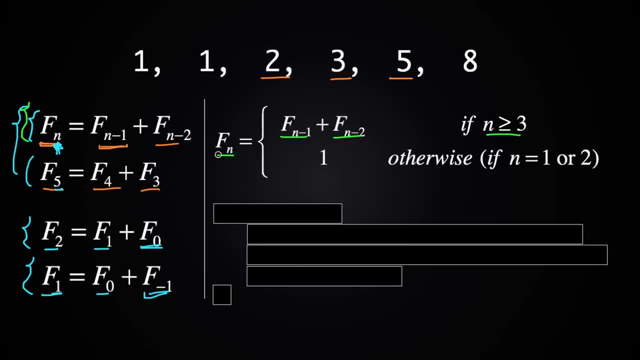 And then the second part will be: Fn is equal to one otherwise, And that's when n is equal to one or two. Now, to solve the problem we saw earlier of writing a function called Fib, we just need to translate this formal definition into code. 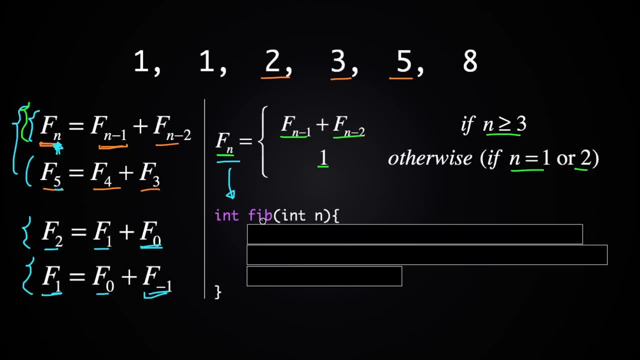 Let's do that. Let's see how we can do that. I just wrote here: int, Fib, int n, And this just means we're going to define a function called Fib, which is going to return an integer, and then it's going to take n. 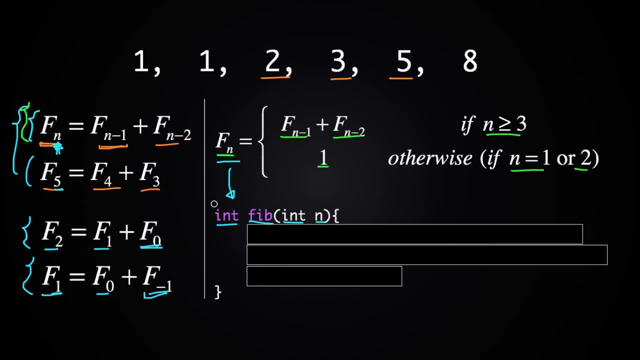 which is an integer as an argument, And then, inside this function, I'm just going to first of all assume that the given n is a positive integer, just for simplicity, And then after that I would say: if n is greater than or equal to three, then return the sum. 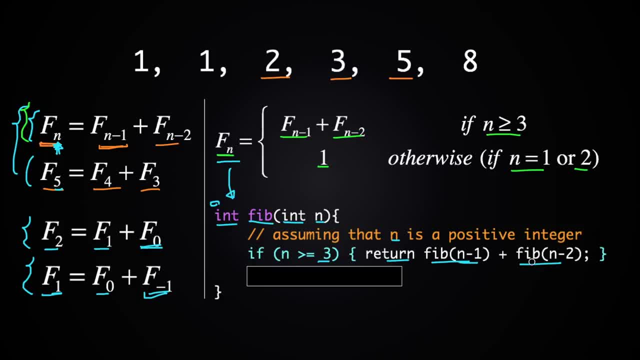 of the two previous Fibonacci numbers, Fib of n minus one and Fib of n minus two, And otherwise n is equal to one or two. So we're just going to return from this function. OK, let's now take a look at a few examples here to see how this function works exactly. 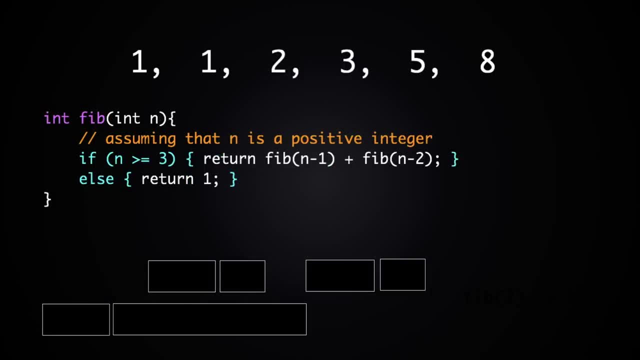 I'm just going to move this function over here. OK, first of all, let's say this function, Fib, is called with three as the argument. Then what happens is we go to this line right here: Three is greater than or equal to three. 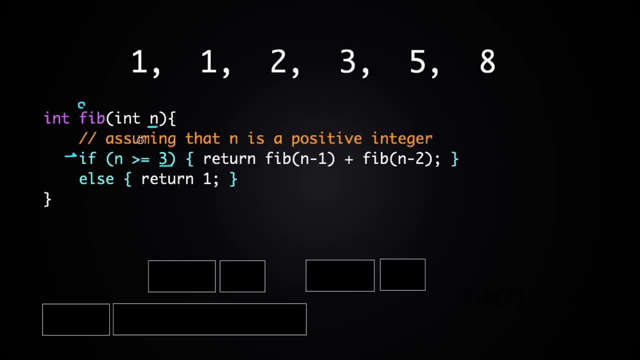 So we'll say, OK, the value, the return value, of Fib of three should be the sum of Fib of one and Fib of two. So that's what I wrote here: Fib of three should be the sum of Fib of two and Fib of one. 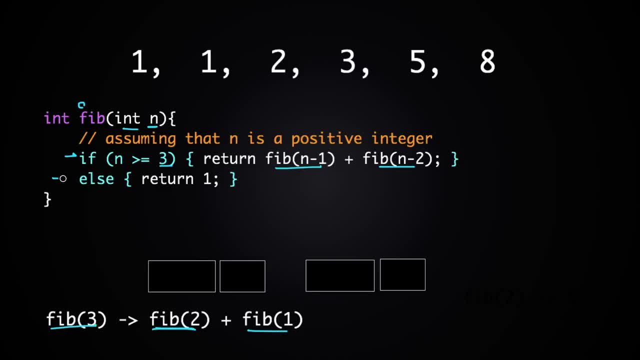 And then in Fib of two, we'll go to this line right here, because two is not greater than or equal to three. So we'll return one from Fib of two, And just like that we're going to return one from Fib of one as well. 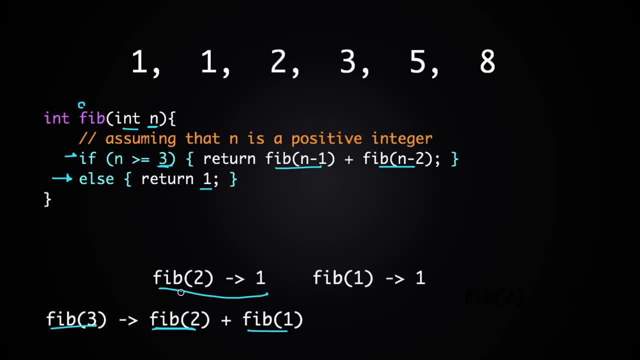 And once we have these two numbers, Fib of two will go in here and Fib of one will go in here. So one will go in here and then one will go in here. So we're going to return one plus one and we're going to return two from our function. 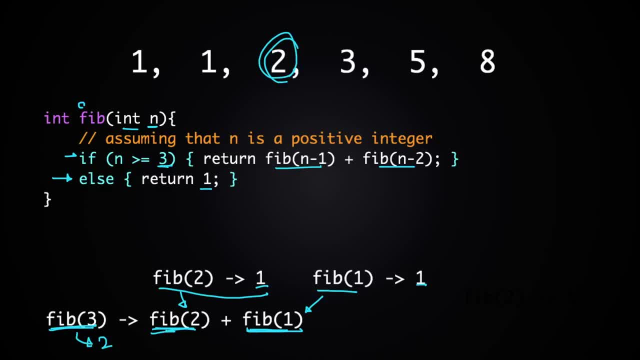 And that's the correct answer. By the way, just quickly about terminology: in a function that uses recursion or in a recursive function, the condition where it doesn't call itself at all but instead returns- for example, just a number- is called a base case. 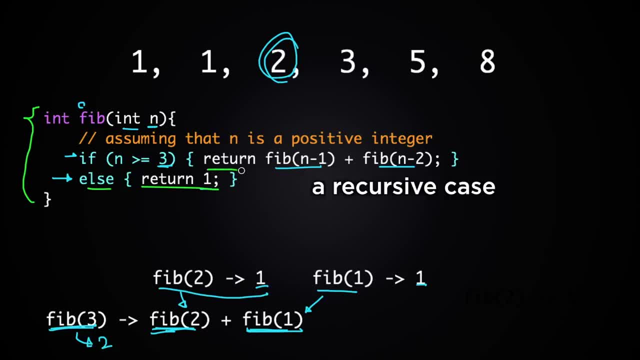 And then the condition where it calls itself is called a recursive case. So in this example, when n is greater than or equal to three, that's a recursive case and otherwise that's a base case. OK, let's take a look at another example here. 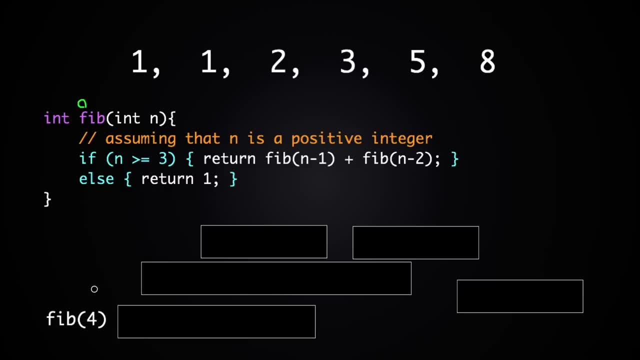 Let's say this function, Fib, is called four as the argument. That's this one right here. Then it goes to this line right here, because n, which is four, is greater than or equal to three. So we want to return Fib of three plus Fib of two as the return value of Fib of four. 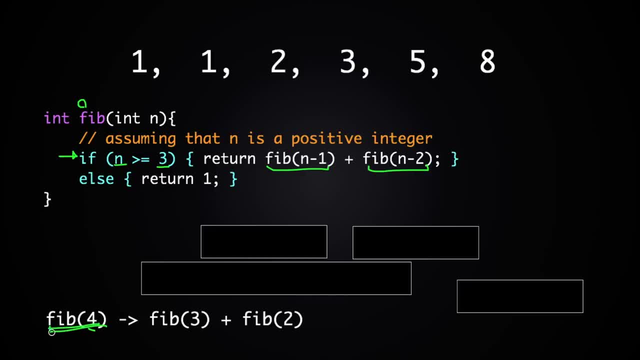 So that's what I wrote here. The return value of Fib of four should be the sum of the return value of Fib of three and the return value for Fib of two, And when we hit that line right here, we don't know what the return value should be for Fib of three yet 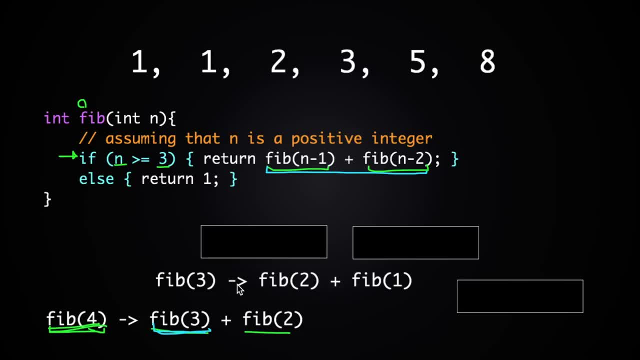 So we'll need to call it separately, and then the same thing will happen. We'll say, OK, whatever we return from Fib of three, that should be the sum of Fib of two and Fib of one. So we'll call Fib of two and then we'll say, OK, the return value for Fib of two. 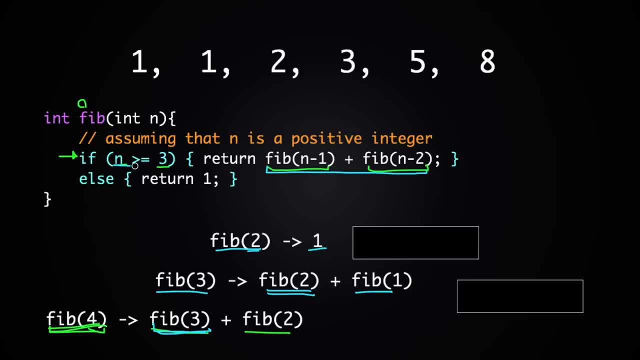 should be one, because two is not greater than or equal to three. So we'll go to this line right here and then we'll return one from Fib of two And then one will go in here and then at this point we'll know that we. 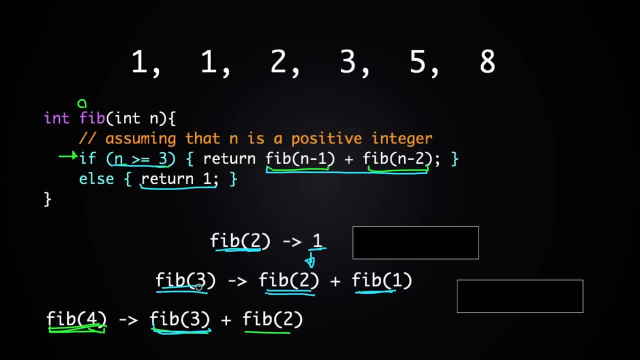 should return one plus Fib of one from Fib of three, And so we're going to call Fib of one, and then it's the same thing. We'll return one from Fib of one, and then one will go in here and then we'll say: 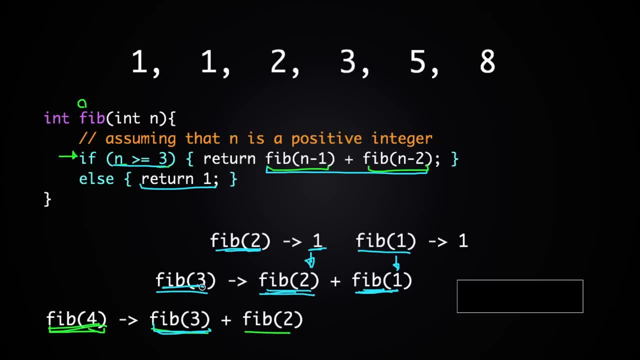 OK, we should return one plus one, which is two from Fib of three. So we'll plug in two right here and then we'll say, OK, we should return two plus Fib of two from Fib of four. But we don't know what the value for Fib of two should be. 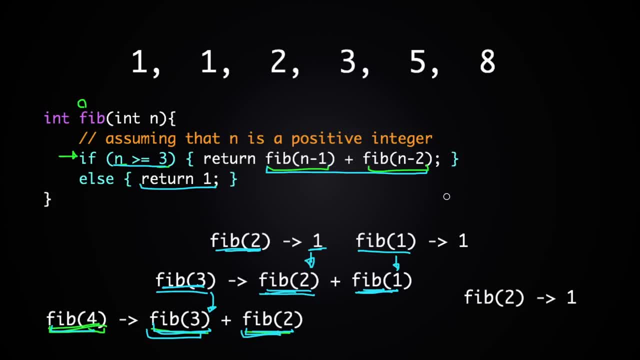 So we're going to call that And then again we'll say, OK, we should return one from Fib of two. So one will go in here and then we have one for Fib of two and two for Fib of three at this point. So we're going to return two plus one from Fib of four, which is three. 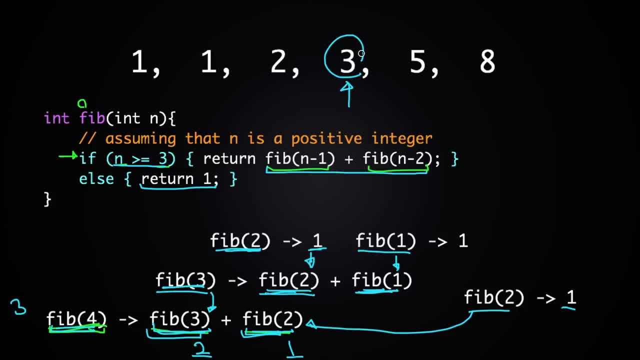 And that's the correct answer, because that's the fourth Fibonacci number. OK, so that's one way to implement this function, Fib, But here you might notice that it's not the most efficient way to do it. To see why it's not the most efficient way to do it and to see how you can fix it: 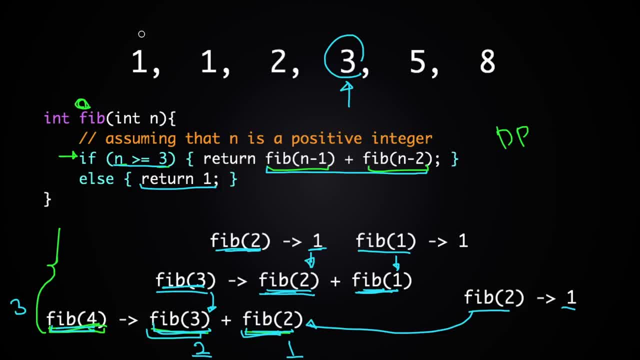 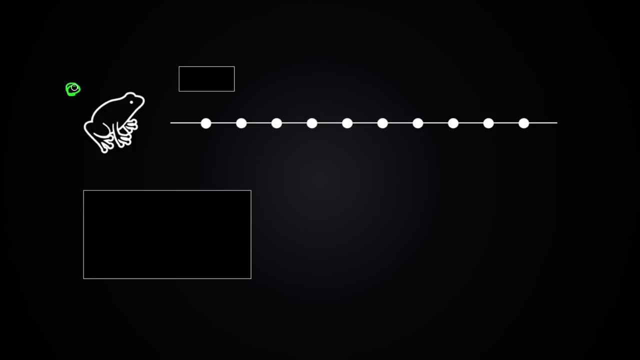 you can just check my video about dynamic programming. OK, and this was number six of my data structures and algorithm series. You can find the entire series in the description below. And to close things off here, let me give you another practice problem for recursion which comes from this video. sponsor: Booleanorg. 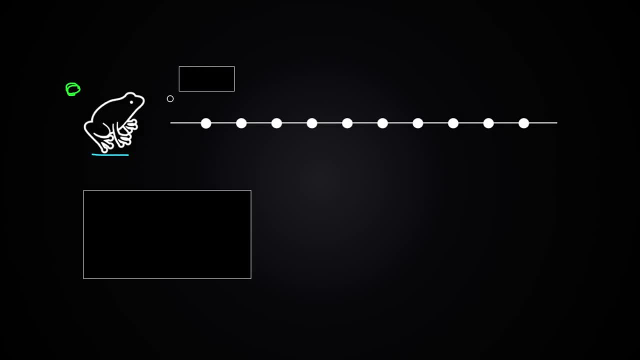 In this problem. there is a frog looking over a river which is 11 feet wide And there are 10 stones placed in this river, one foot apart. So from the end of the river- the beginning of the river, I guess- to the first stone, that's one foot. 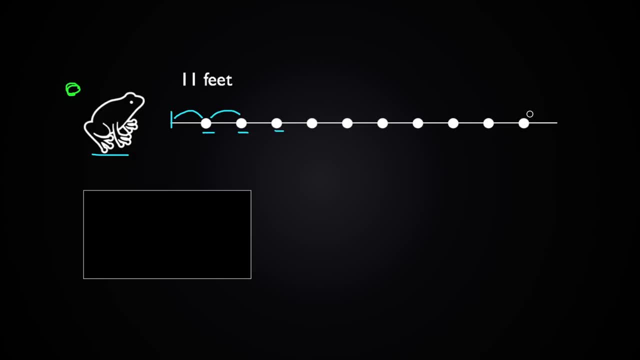 And then to the next stone- that's one foot, and so on, And then from the last stone to the end of the river, that's one foot as well, And then this frog is able to jump either over one foot or two feet. So the first step this frog could make is 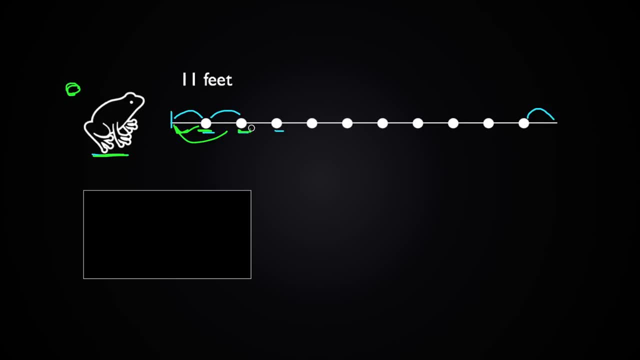 either to this stone right here or this stone over here, And if the frog decides to go to this stone, then it can jump to this stone or to this stone over here. And the question here is: how many ways are there for this frog? 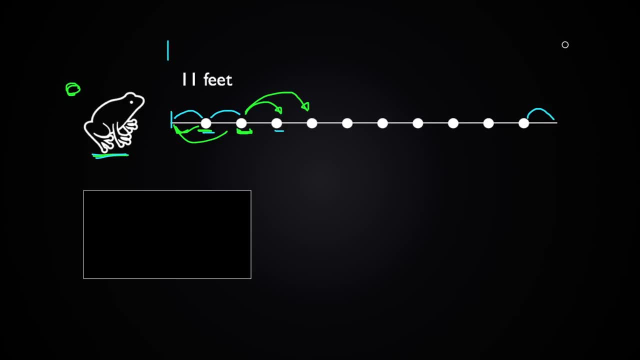 to jump from this side of the river to that side of the river And note that this frog can never go backwards. And a simpler version of this problem would be this one, right here, where there's a frog on one side of the river, just like before. 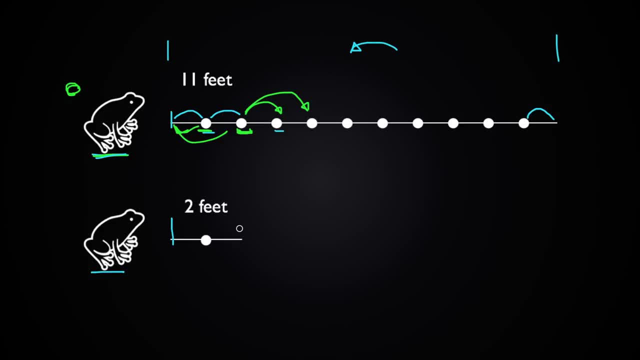 But instead of 11 feet, this time the river is only two feet and there's only one stone placed. So in this example, there are only two ways for this frog to go from this side to that side, because the first way would be to jump. 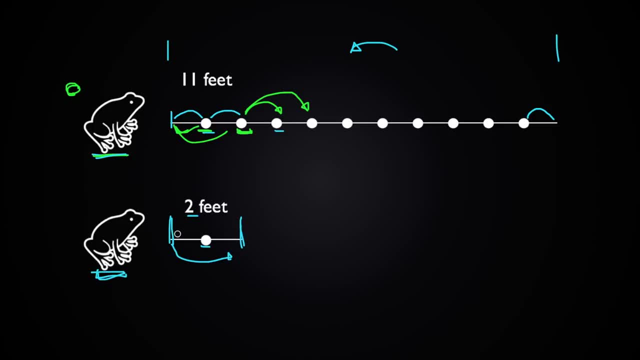 directly from this side to that side, and then the second way would be to jump to the stone and then to the other side, To that side of the river. So see if you can solve the same problem for the case where the river is 11 feet wide instead of two feet wide. 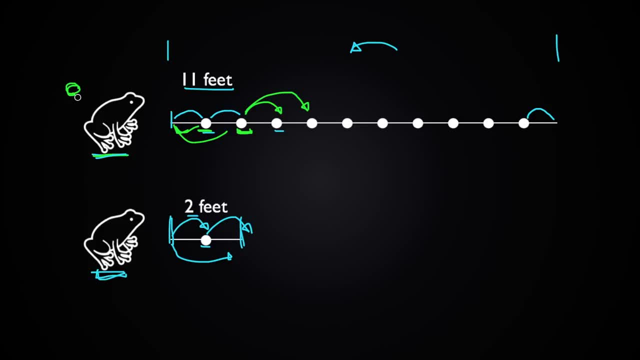 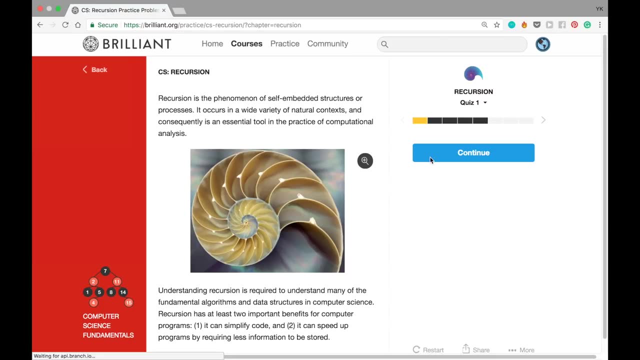 And actually the solution is pretty interesting and it involves using recursion. Now, Brilliant is a website where you can practice your problem solving abilities with interesting problems like these, and that's really the best way to learn. So if you want more interesting problems, 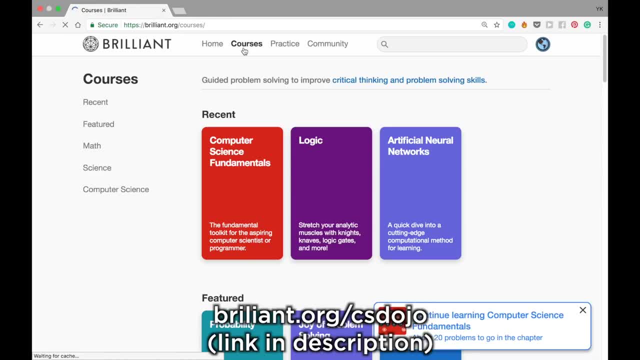 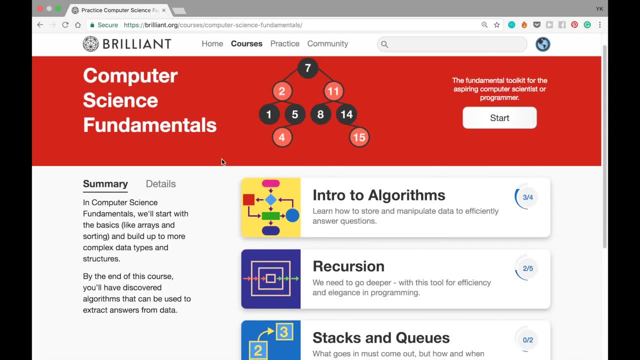 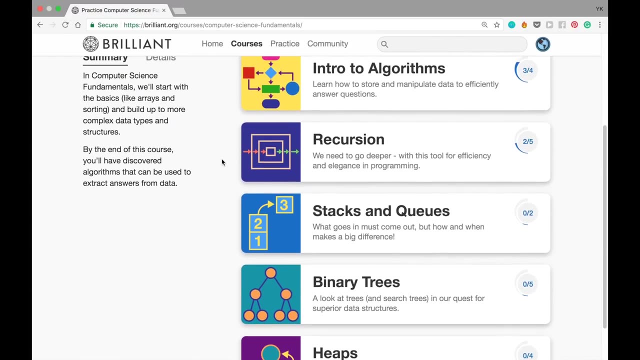 about data structures. just go to brilliantorg slash CISdojo and maybe check out their computer science fundamentals course. There you'll be able to find more interesting problems about topics like algorithms, recursion, stack and queues and so on, And there you'll be able to find the solution to the frog problem as well. 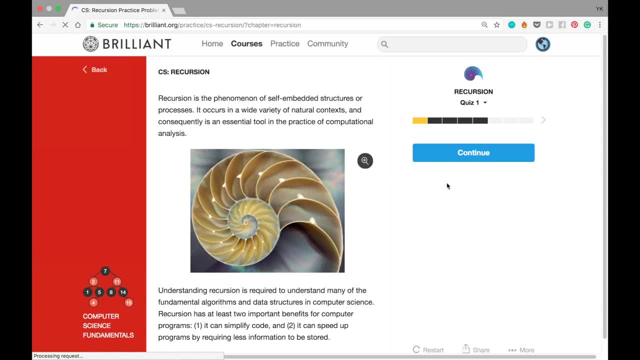 OK, thanks for watching this video and I'll see you in the next one.